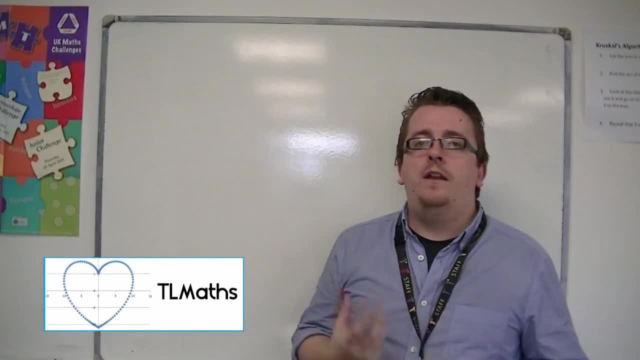 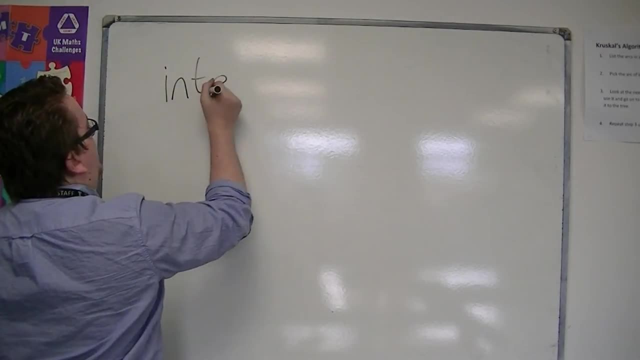 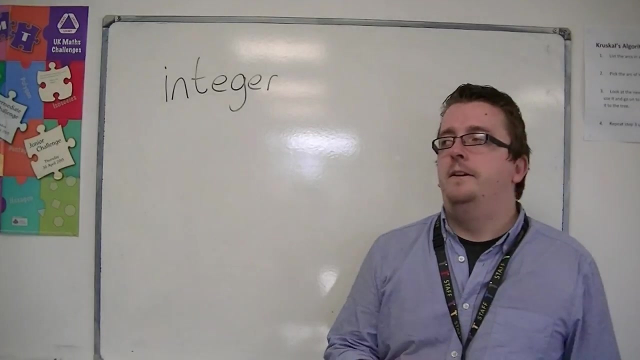 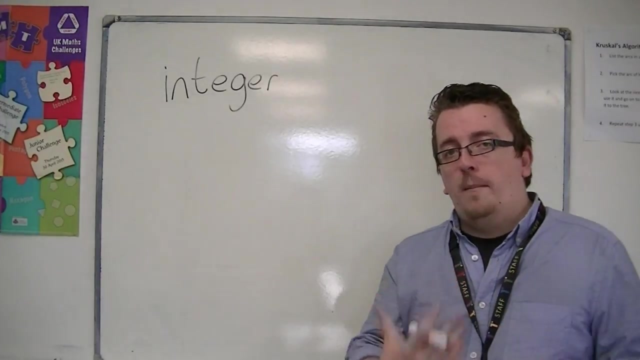 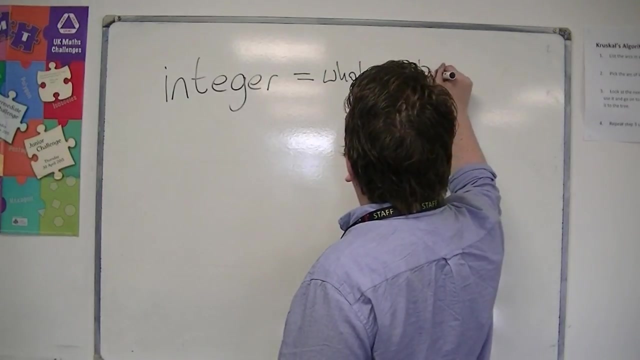 Now you could be asked to round a number to the nearest integer And the word is spelt I-N-T-E-G-E-R, And some people pronounce integer mistakenly. So this is integer And an integer is a whole number. It is the special maths-y word for whole number Or unit. 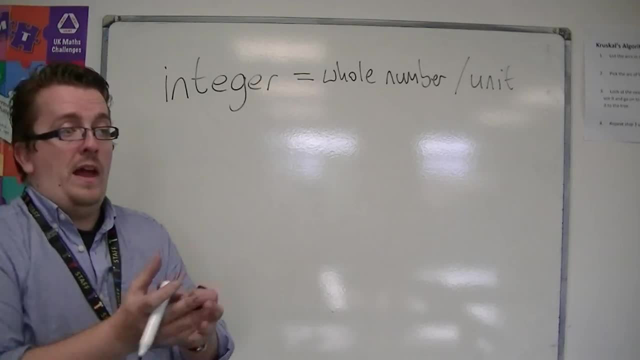 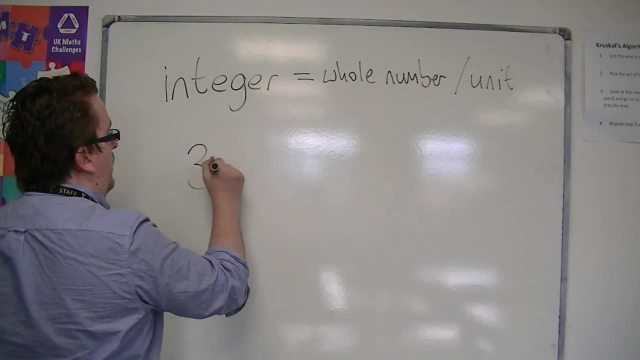 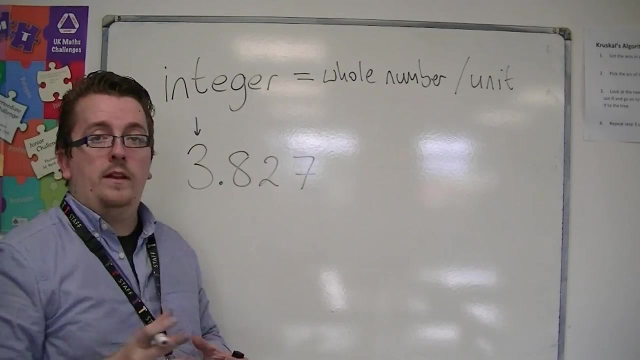 So unit is that place value where we are one to the left of the decimal point. So if I look at the number 3.1.. 8,, 2,, 7. Then this was the units column. So if you go back and you look at the video that I made right at the beginning, 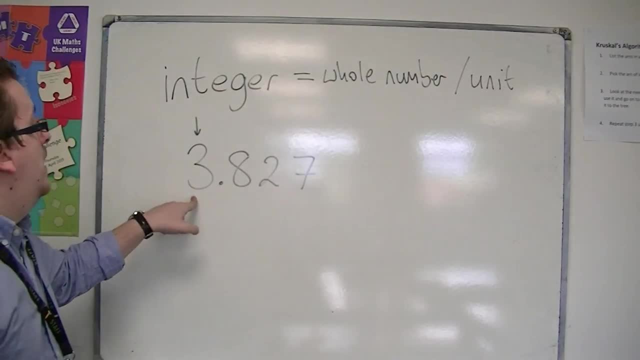 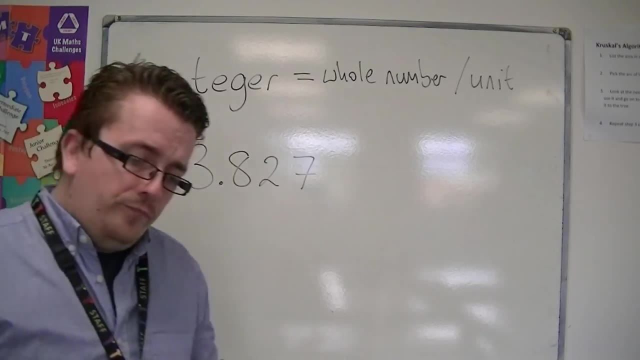 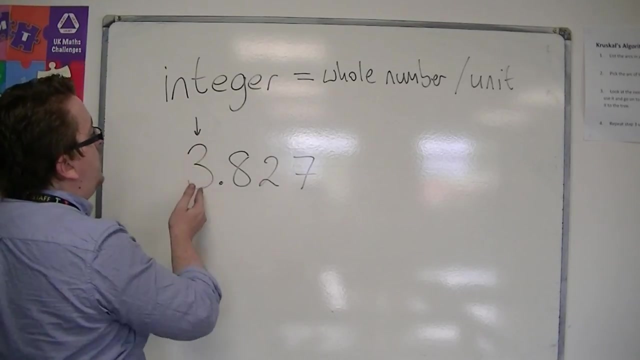 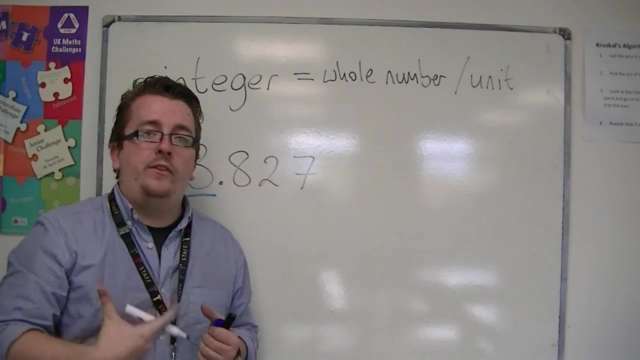 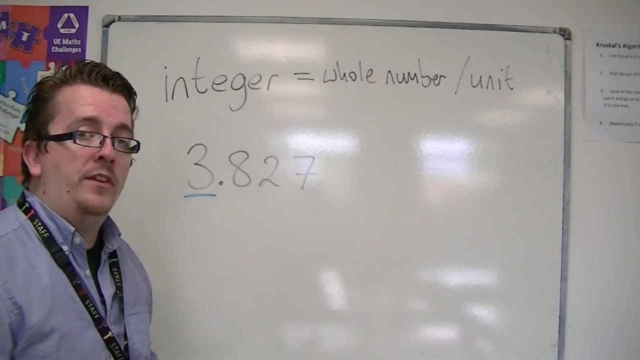 Then we looked at place value. This is the units column. These are where we are looking at the whole numbers. So what we want is: if I am going to round this to the nearest integer, Then this is the units column And in all the ways, in all the same cases that we have been looking at before we identify the place value that we are considering. 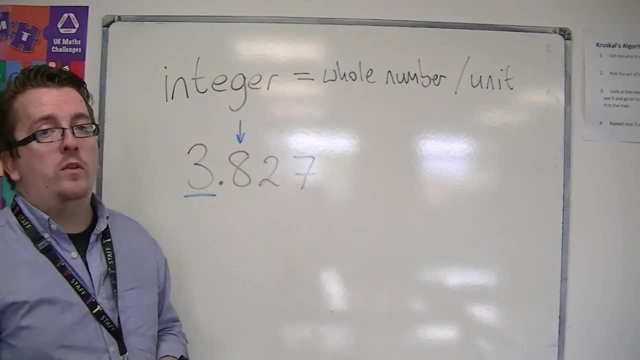 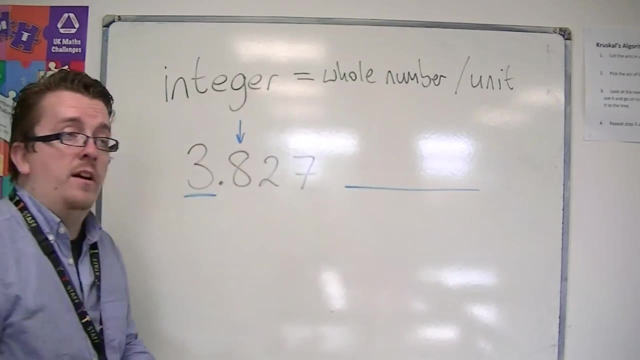 We look one to the right, and that will determine whether we should round up or round down So effectively. what I have done is I have split my number line up into units, So I have 2,, 3,, 4,, 5,, 6,, 7, etc. 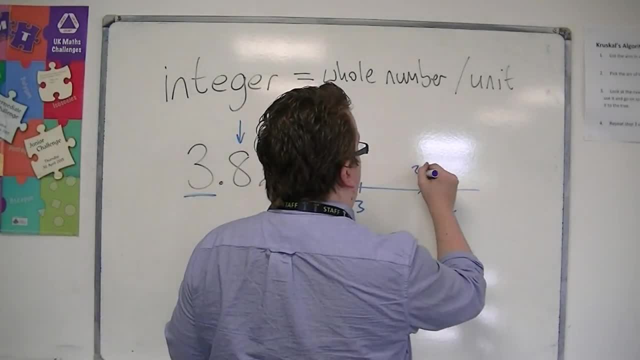 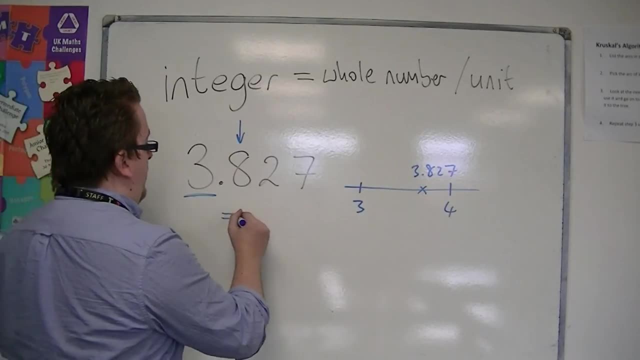 And 3.8.. 8,, 2,, 7 is roughly about here, So that 8 is telling me that I need to round up, So I would round this to 4, to the nearest integer. I have got a very squeaky pen. 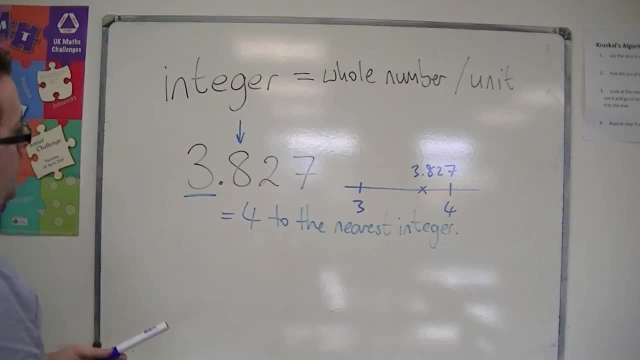 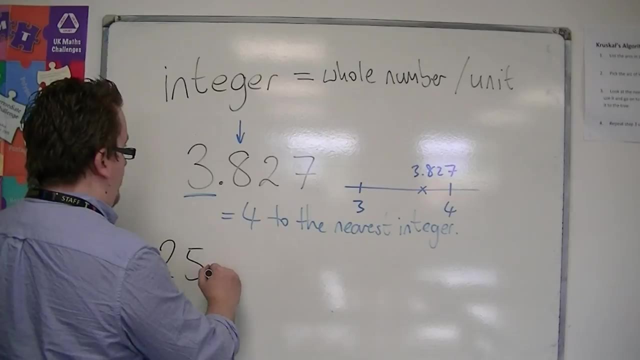 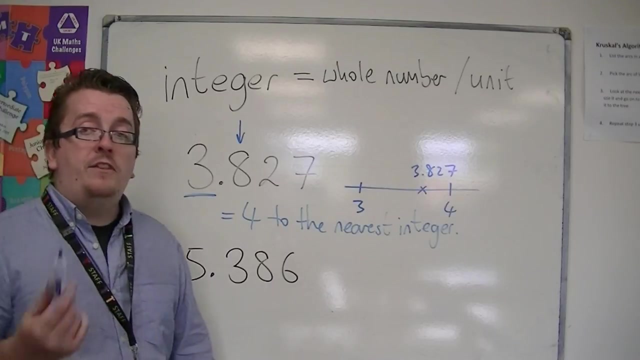